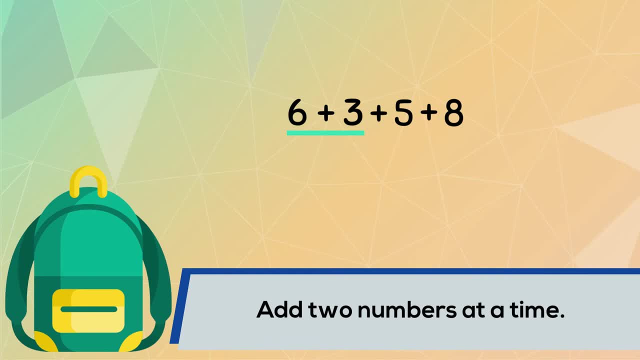 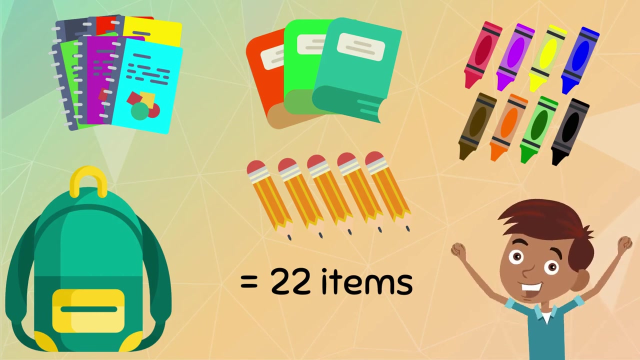 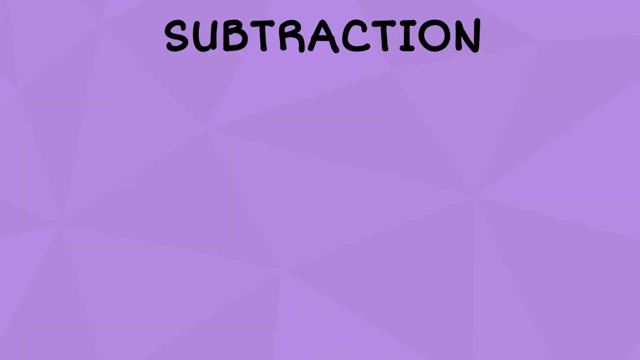 Six notebooks plus three textbooks equals nine items. Five pencils plus eight crayons equals thirteen items. So now we just add nine plus thirteen, which equals twenty-two items. Paul has twenty-two items in his bag. No wonder it's so heavy. Now let's practice subtraction using these two rolls of ribbon. 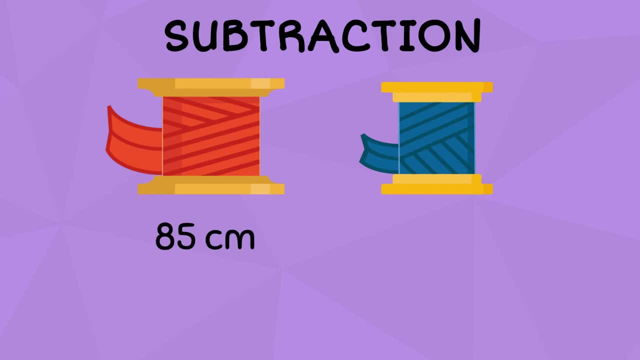 The first roll is eighty-five centimeters long. It's all rolled out. The second roll is sixty-three centimeters long. It's all rolled out. What is the difference between the length of the two rolls? Remember, in math that the word difference means the result of subtracting one number from another number. 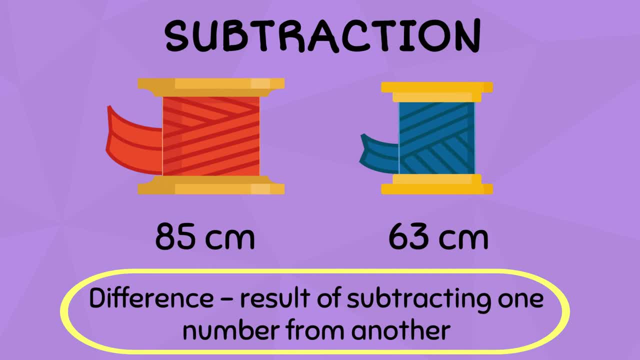 Remember in math that the word difference means the result of subtracting one number from another number. So how would you write this subtraction sentence? Did you say: 85 centimeters minus 63 centimeters? That's correct. Now the easiest way to do this is by writing the numbers so that the place values are lined. 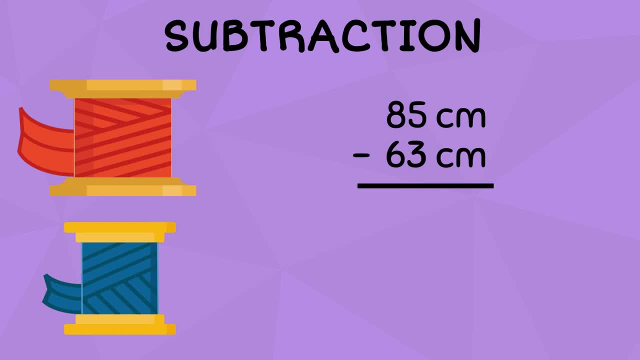 up in columns, Then just subtract them, starting with the numbers in the ones place, Starting with the ones we have. 5 minus 3 equals 2.. Make sure you write the answer under the ones column. Then continue with the tens. 8 minus 6 equals 2.. 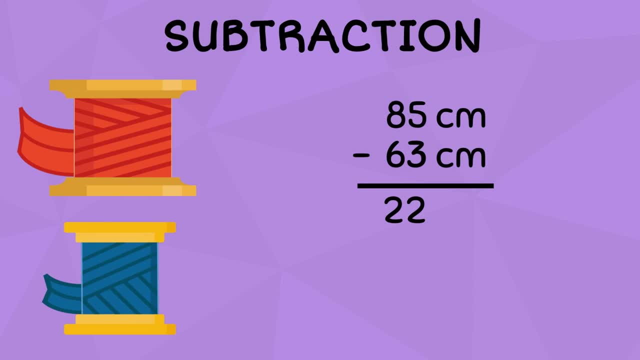 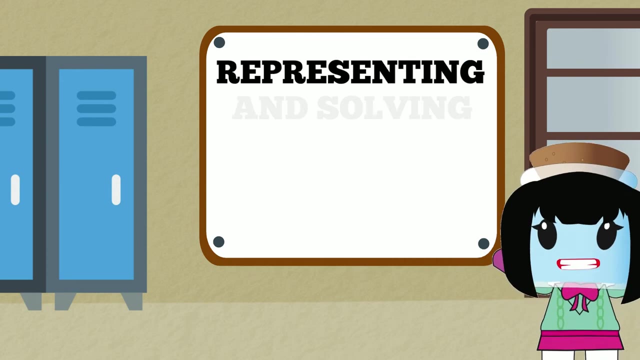 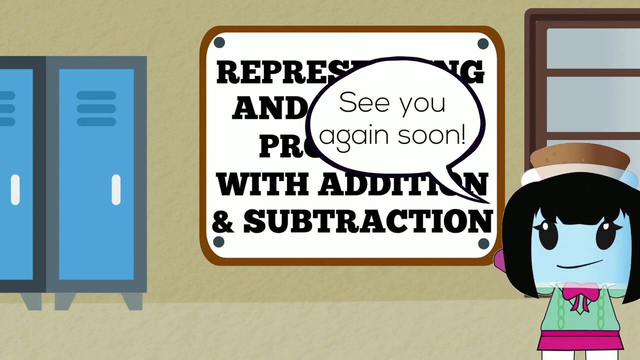 Okay, So the difference between the lengths of the two rolls of ribbon is 22 centimeters. Great job. I hope this has helped you learn how to represent and solve problems with addition and subtraction. See you again soon. Bottle Learning is making math fun and motivating.